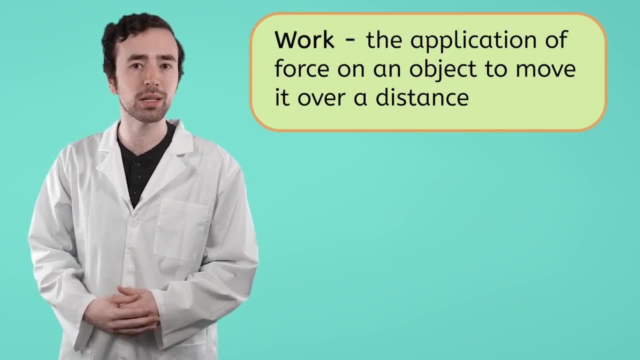 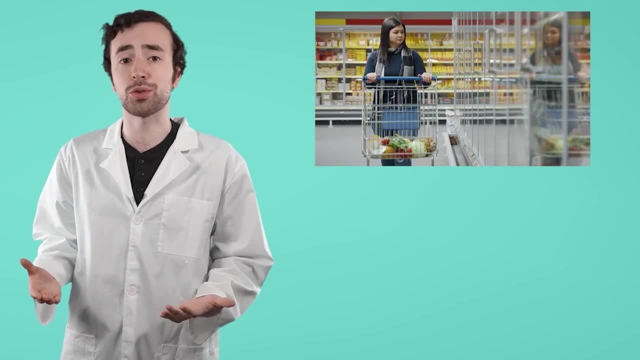 else. Work is exerting a force on an object and causing it to move a certain distance. So if you've ever pushed a shopping cart at your grocery store, you were doing work. If you ever picked a weight up off the ground, that's also work. 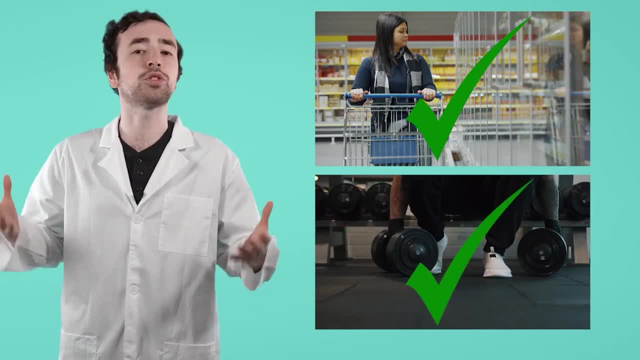 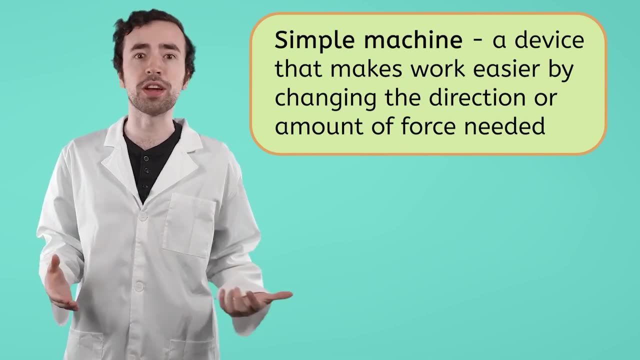 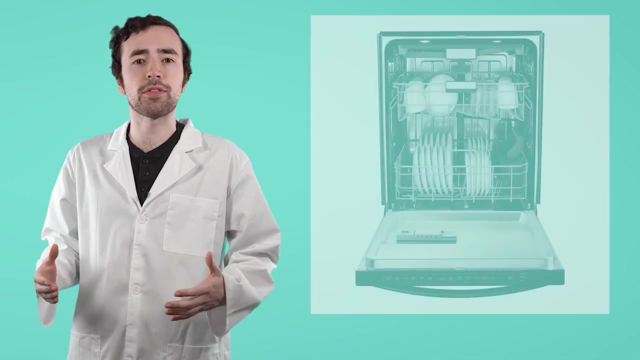 You were exerting a force on an object and causing it to move a certain distance. So simple machines make work or moving things easier. But what is a simple machine exactly? When I said machine, you might have thought about a dishwasher or a car you know. 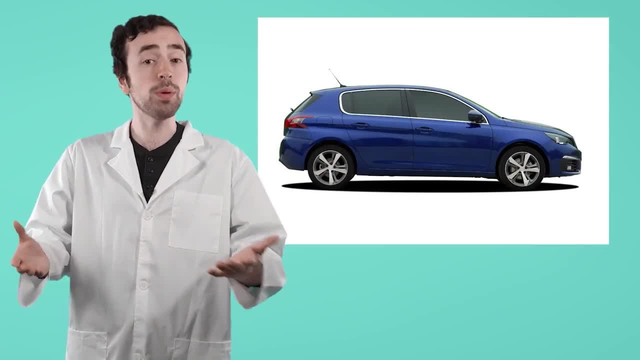 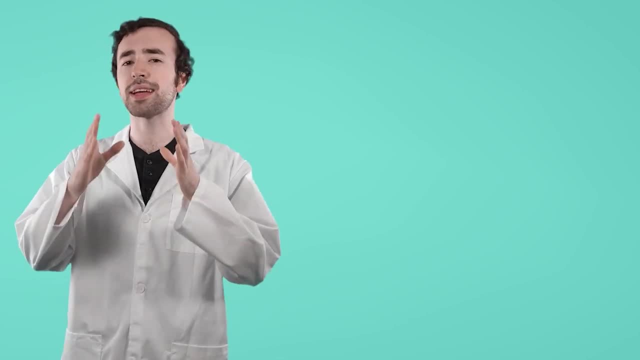 something with an engine and a lot of moving parts, And you'd be right, Those are machines. But machines don't have to be that complex. All a machine, what it is, is something that directs force, And simple machines are just that simple. 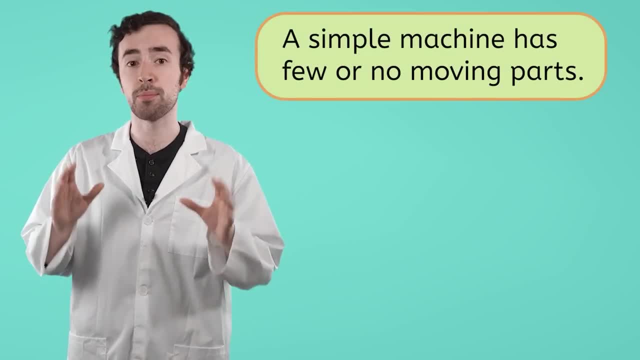 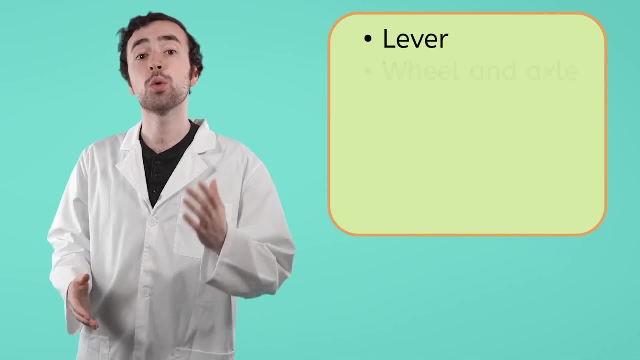 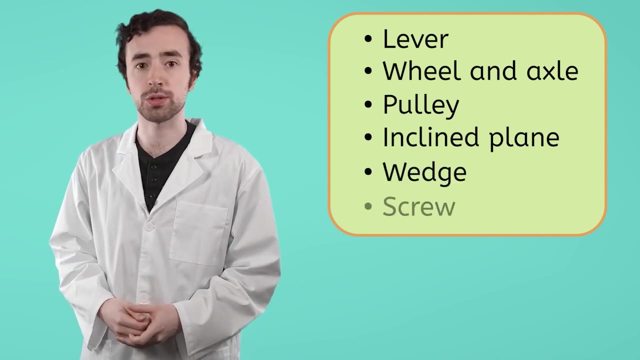 They're machines with very few or no moving parts. For our purposes, there are six different types of simple machines: Levers, wheels and axles, pulleys, inclined planes, wedges and screws. To get a better understanding of what simple machines are and what they do, let's take a 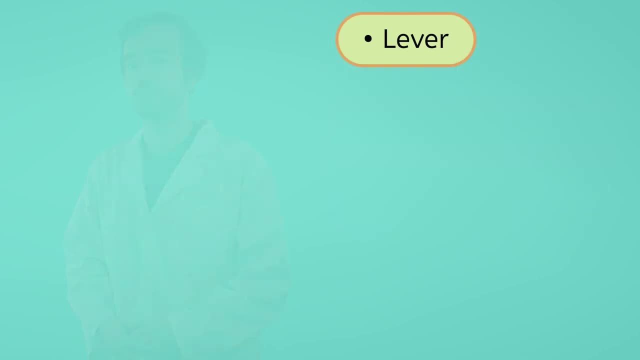 closer look at that first type of machine. And that's what we're going to do. We're going to take a closer look at that first type: levers. A lever has two main parts: a beam and something it rests on called a fulcrum. When you push down on one end of the beam, it pivots or rotates. 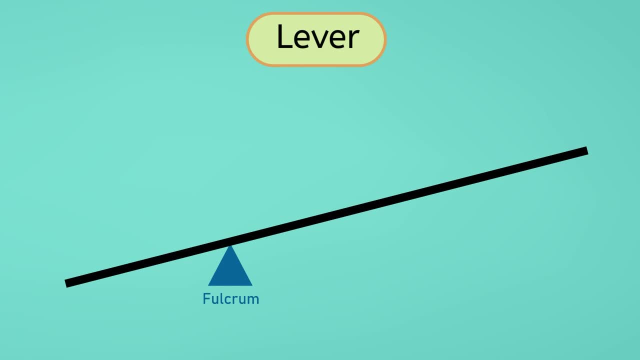 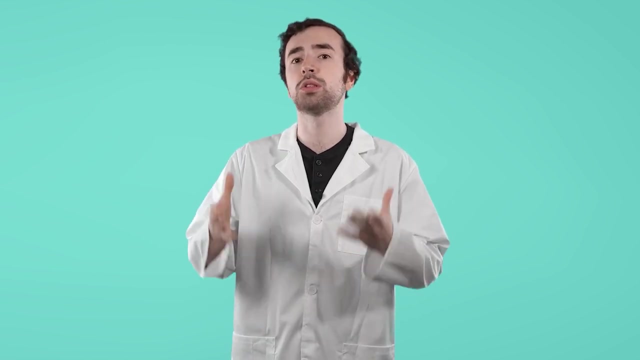 along the fulcrum and the other end will move upward. Your push is called effort and the side that's lifted is called the load. Levers allow us to lift heavy objects. We can lift heavy objects. We can lift heavy objects. We can lift heavy objects or loads much easier. A great example of a lever that you're probably 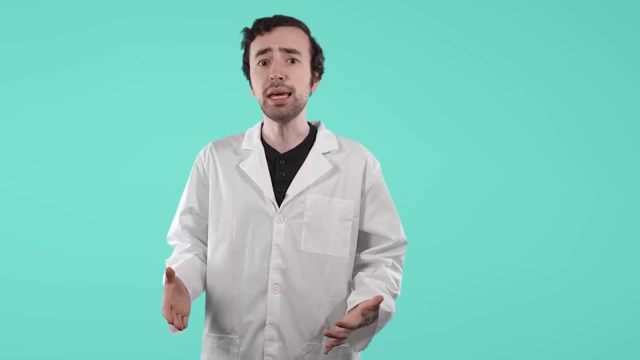 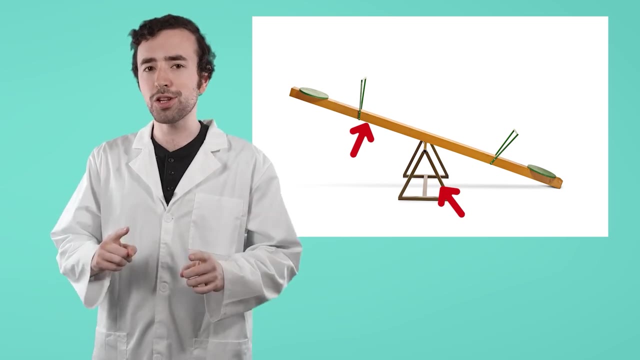 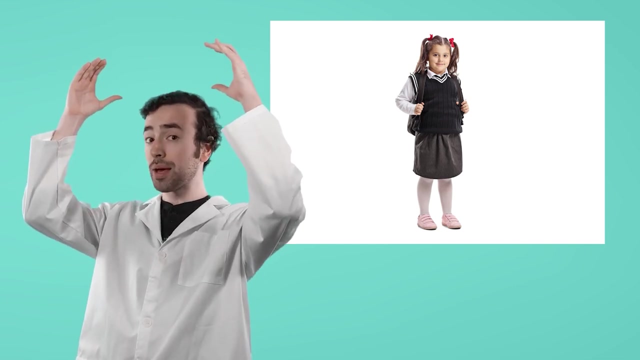 familiar with, especially if you've spent a lot of time on playgrounds, is a seesaw. A seesaw is a lever because it has a beam and a fulcrum. Imagine trying to pick up your friend and lift them over your head. You might be able to do it, but it would take a lot of effort and 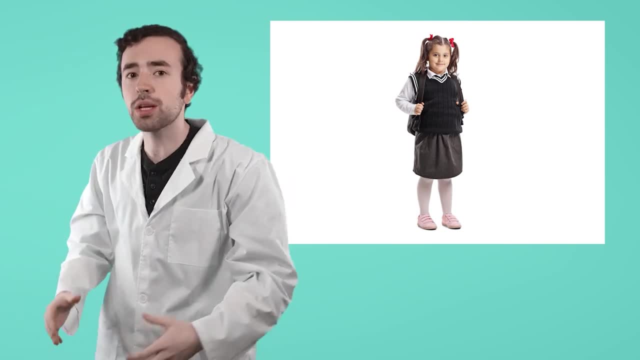 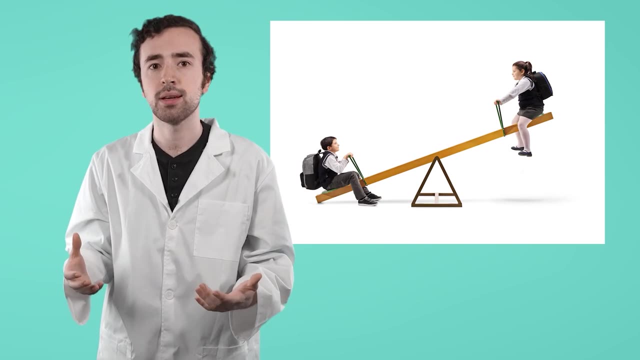 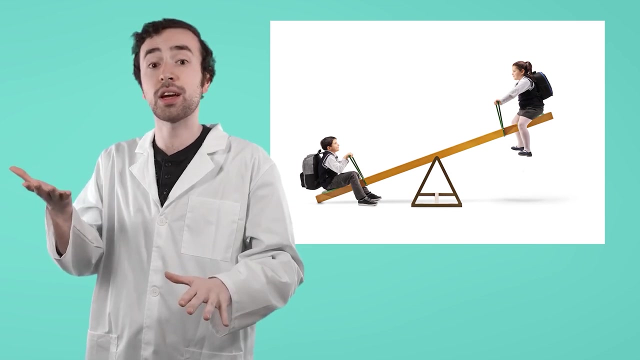 you'd have to ask them nicely. But with a seesaw you could get a lot of effort and you'd have to get that same result: your friend being lifted into the air just by sitting down on the other end. The lever allows us to change the direction in which the force is applied, giving us our 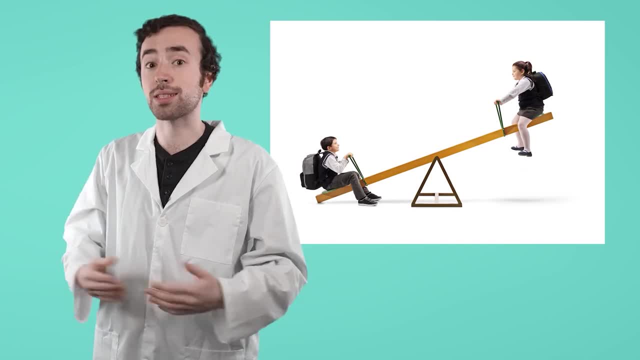 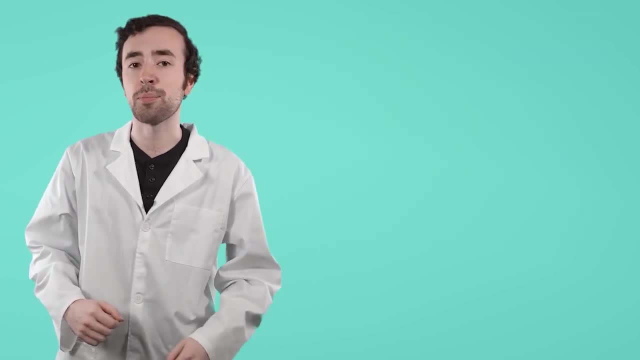 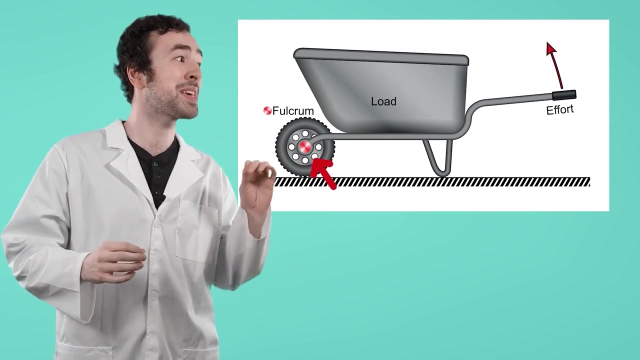 desired outcome much easier. Your friend still gets sent in the air and you put in a lot less effort to do it. Another great example of a lever that you know about is a wheelbarrow. Now, this is different, because the fulcrum is on the ends and the load goes in the middle. Also, instead of 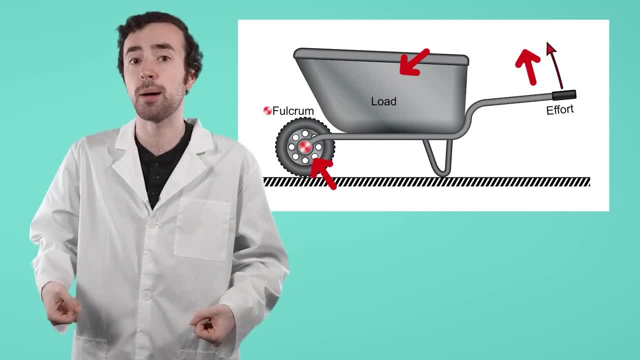 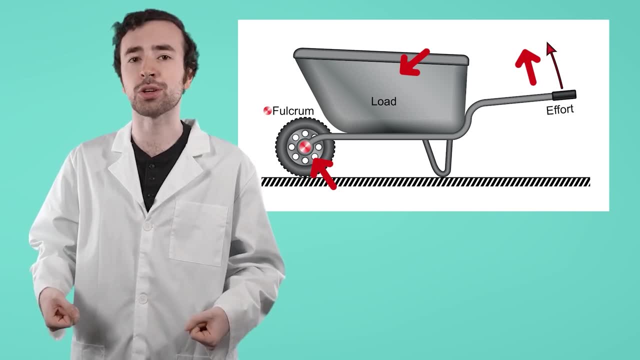 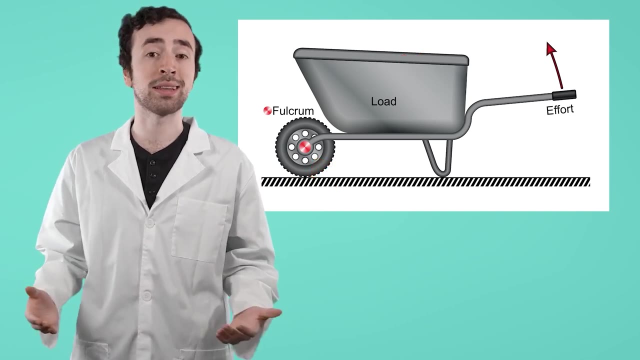 our effort pushing down, we lift the wheelbarrow up and the load comes up with us. The wheelbarrow allows us to lift objects much easier than without one. Seesaws and wheelbarrows are far from the only levers we use in our day-to-day lives. Once you know what to look out for- beams and fulcrums. 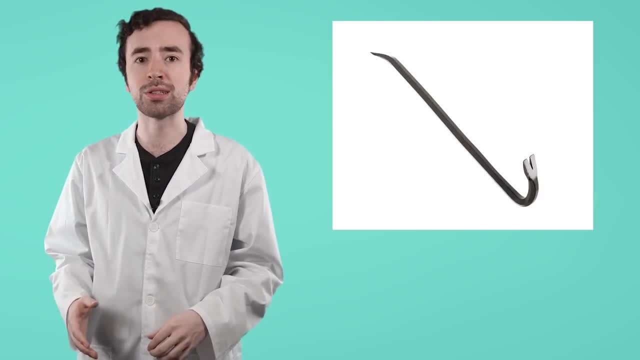 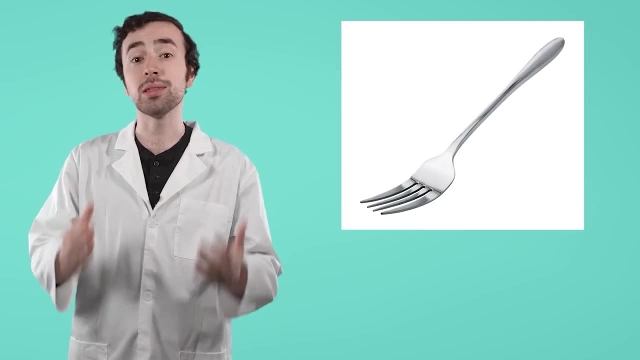 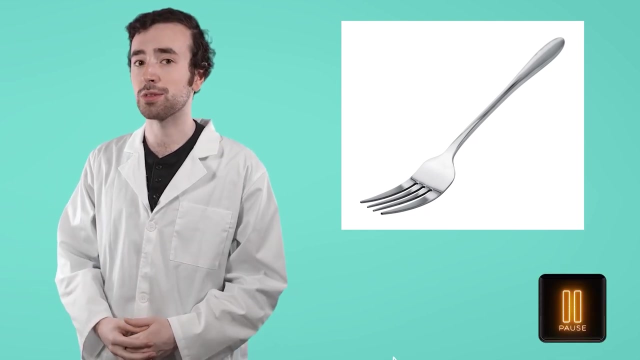 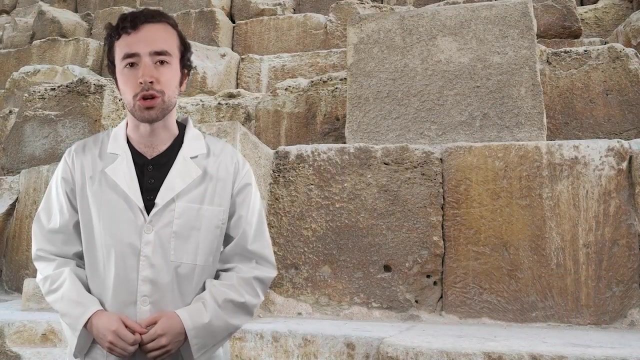 you will notice levers everywhere: Crowbars, scissors, those little handles you use to flush toilets, even forks are all levers. Can you think of some other examples of levers? Pause the video here to jot down your thoughts in your guided notes. Archaeologists have determined that the ancient Egyptians used levers when they 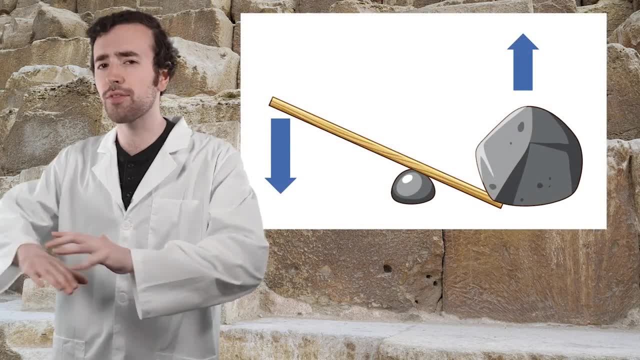 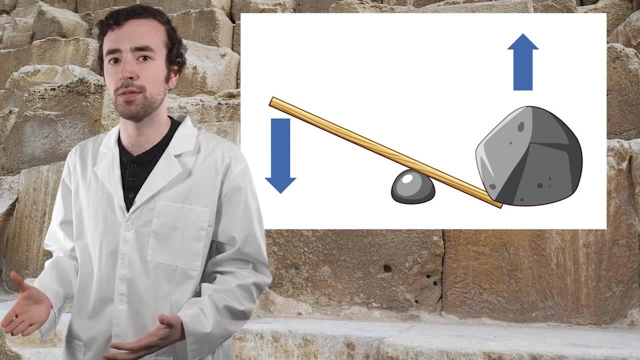 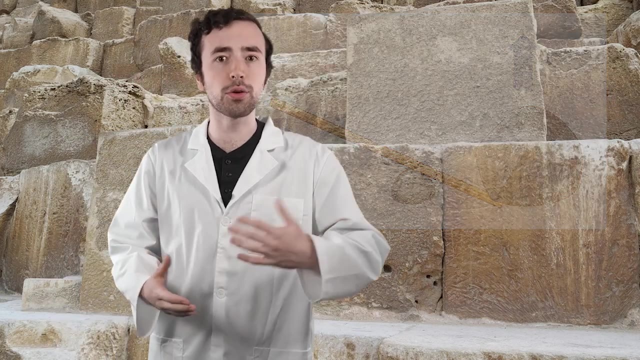 were constructing the Great Pyramids, They used levers to pry the heavy stones out of the ground. There's no way they could have lifted them themselves, but the levers made the work much easier. The Egyptians also used other simple machines like 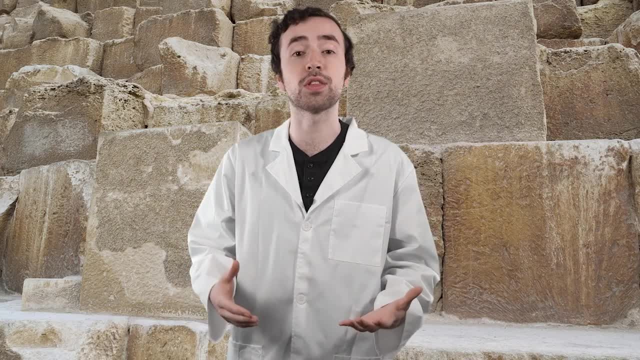 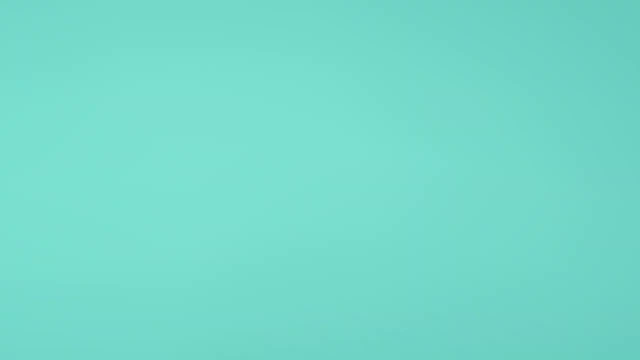 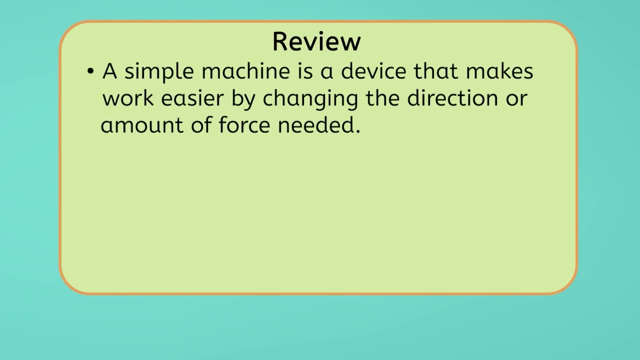 wedges and pulleys to transport and lift the stones when they were building the pyramids, but we'll learn more about that in future lessons. Those ancient Egyptians were pretty clever. Let's review everything we've learned today about simple machines. A simple machine is a device that makes work easier by changing the direction or amount.